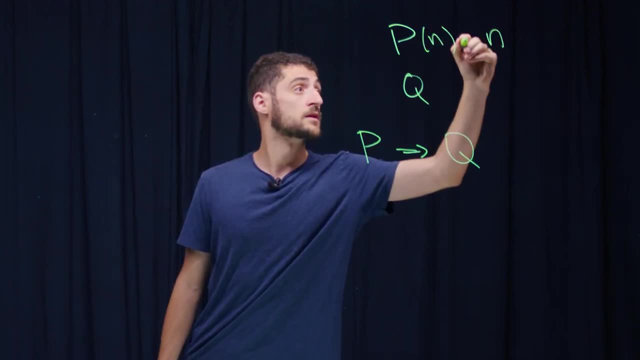 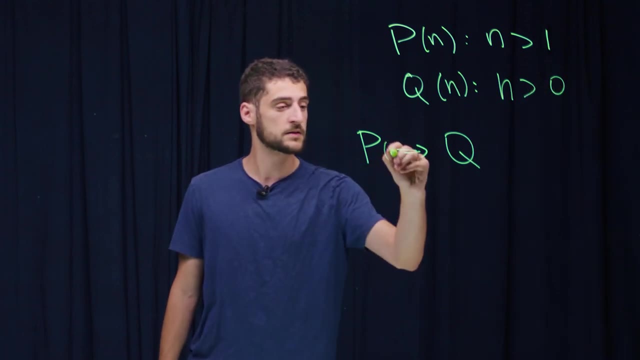 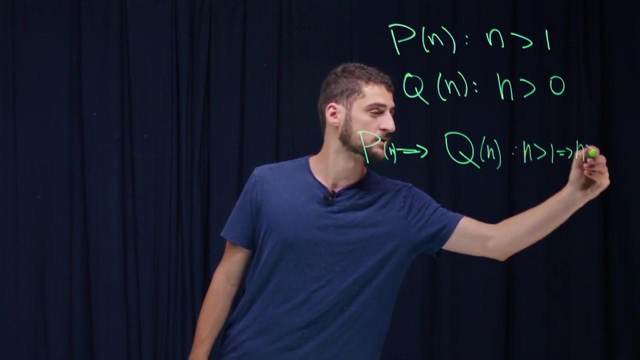 Let's consider some example. p of n be a statement that n is greater than 1,. q of n be a statement that n is greater than 0. In this case, p of n implies q of n state that if n is greater than 1, it means that n is greater than 0. It's easy to see. 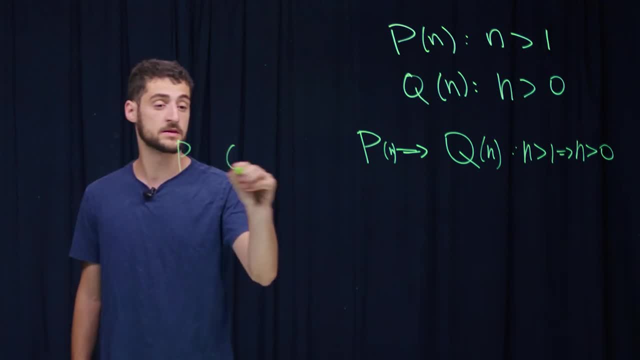 that it's always true. Let's consider some cases. If n is less than or equal than 0, then p is false. q is false as well. If n is equal to 1, then p is greater than 0. If 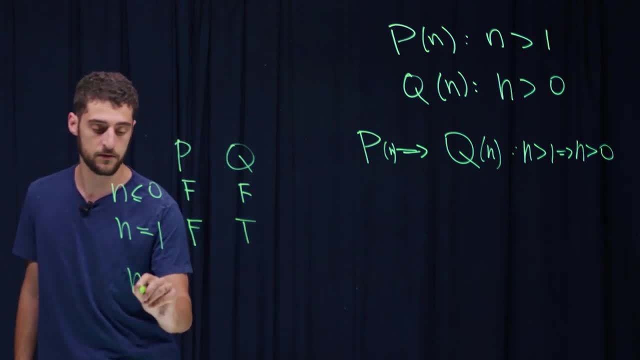 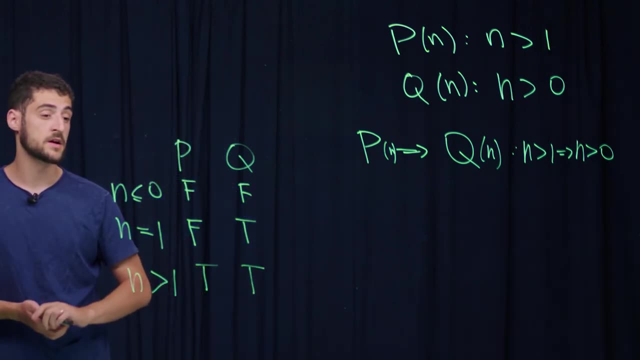 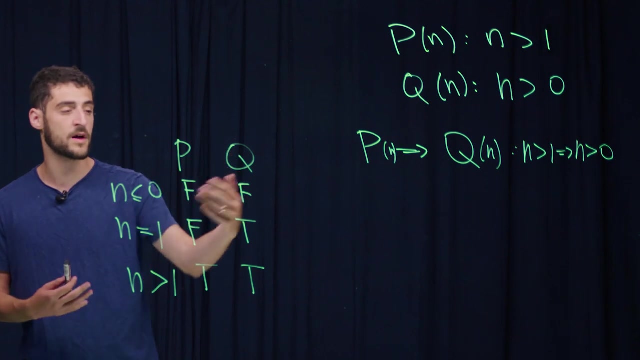 q is still false, but q is true. And finally, if n is greater than 1, then both of them are true. This table said that if p is true, q should be true as well. However, if p is false, then it doesn't matter. what is the truth value of q? Now let's try to extract. 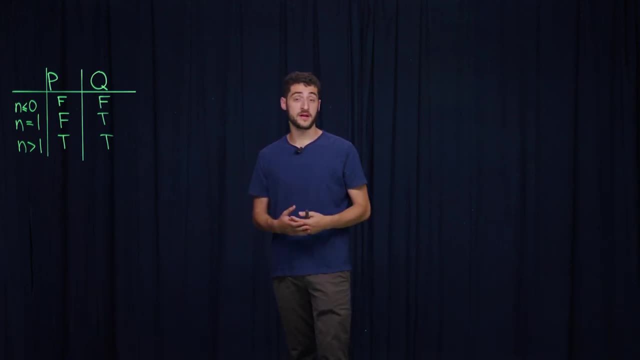 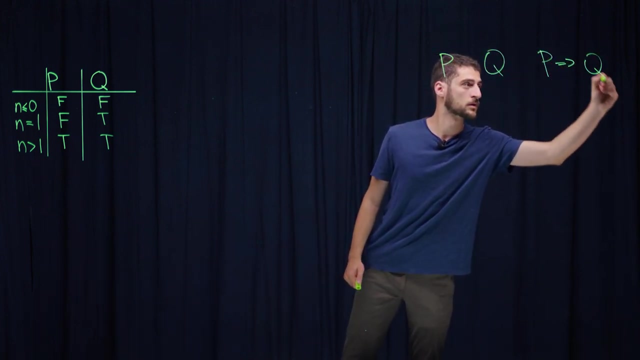 some data from this table to define formally the implication. So we have a statement p, we have a statement q and we have a statement p, So p implies q. If p is true, then to make this implication true, q should be true as. 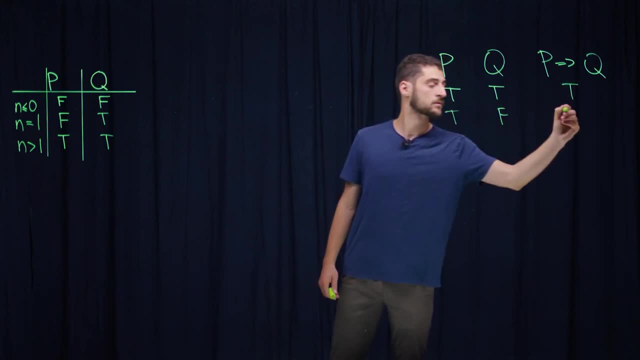 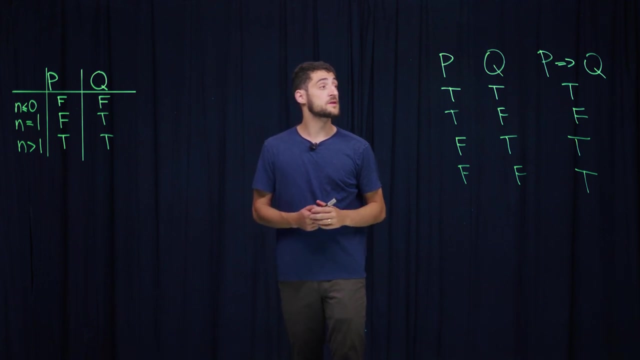 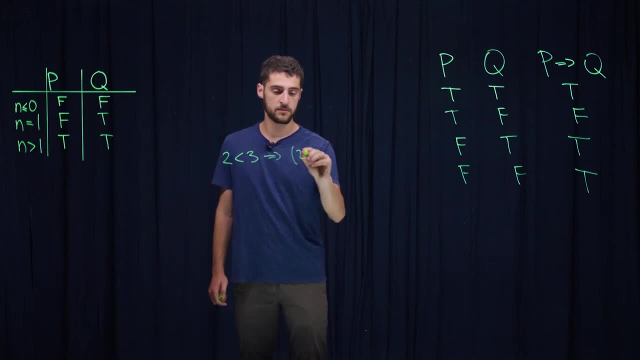 0.. 3 is less than 3 implies 2 times 2 is equal to 4, or 3 less than 2 implies 2 times 2 is equal to 4.. And in mathematics they make sense. However, in real life they sound.